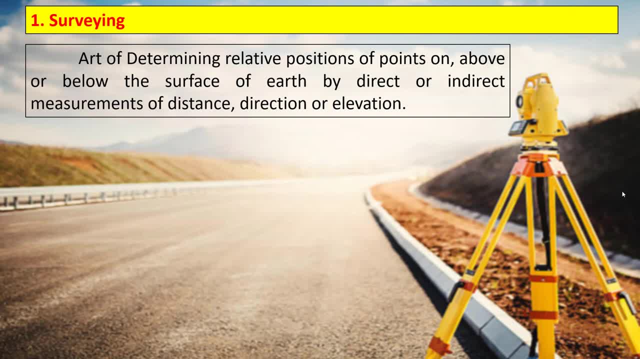 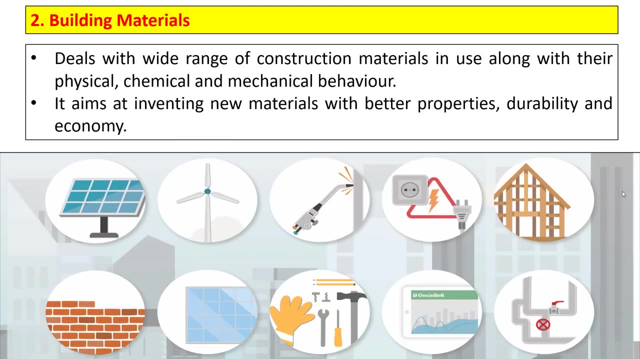 obtained by taking measurements in the vertical plane, termed leveling. The surveying can be classified into plane surveying and geodetic surveying. Next we have building materials. It deals with wide range of construction materials in use, along with their physical, chemical and mechanical behavior. Also, it aims at 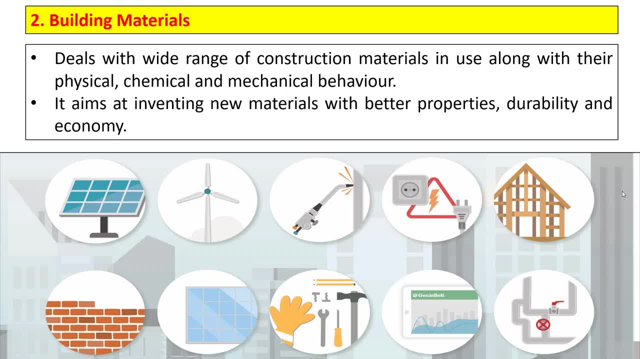 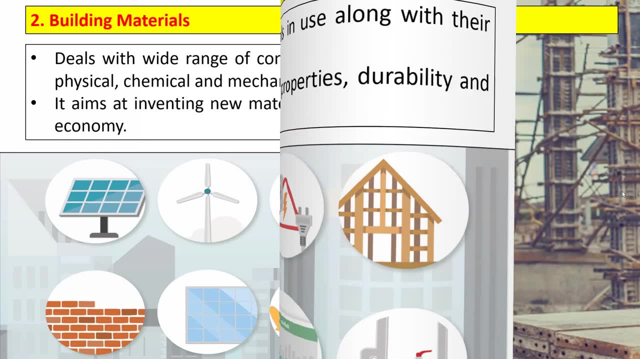 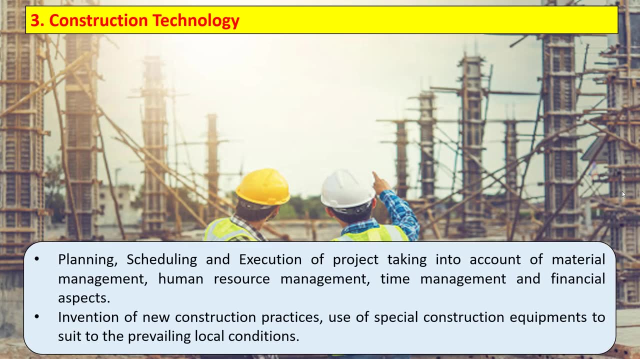 inventing new materials with better properties, durability and economy. Next one is construction technology. It deals with planning, scheduling and execution of the project, taking into account of material management, human resource management, time management and financial aspects. It also deals with invention of new construction practices, use of special 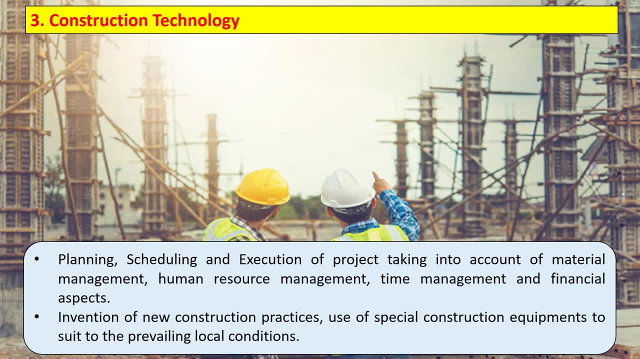 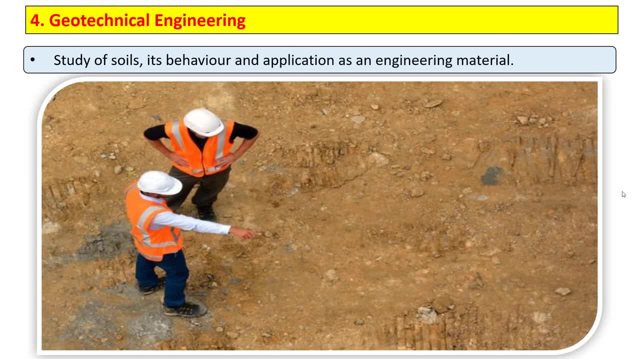 construction equipments to suit the prevailing local conditions. Next we have geotechnical engineering. Mainly it deals with study of soils, its behavior and application as an engineering material. We can also say that this branch of civil engineering is also called soil mechanics. It is a discipline of civil engineering in which the study of soil 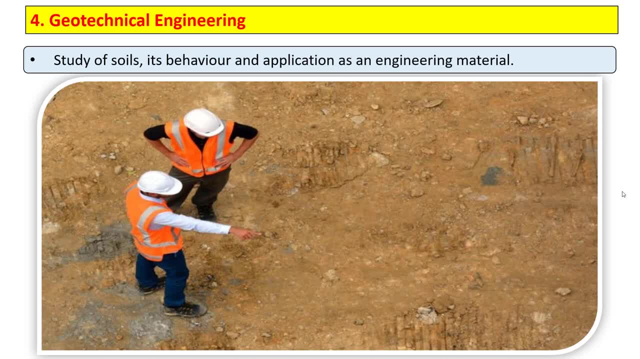 its behavior and application of load and its use as an engineering material in the construction of earthen dams is done. The properties and strength characteristics of soil are studied in this subject. The knowledge of this subject is useful in the design of earthen dams, different file foundations, buildings foundations, etc. Next we have structural. 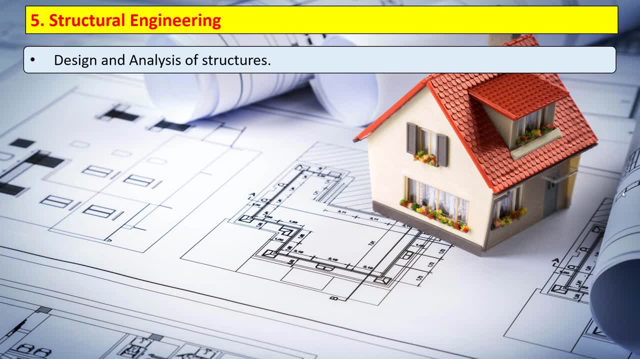 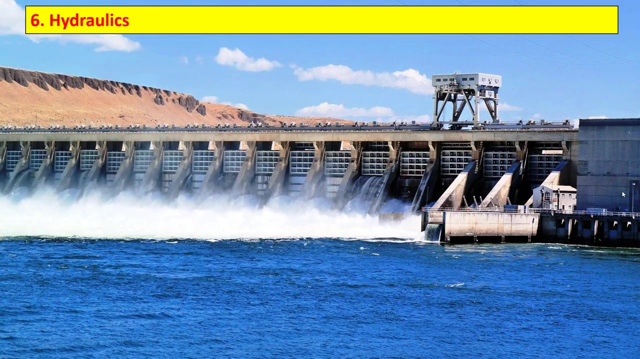 engineering. Structural engineering mainly deals with the design and analysis of the structure After planning. the most important thing the civil engineer has to do is the design and analysis of the structure for its safety and structural integrity. Next we have hydraulics. It deals with the practical aspects of 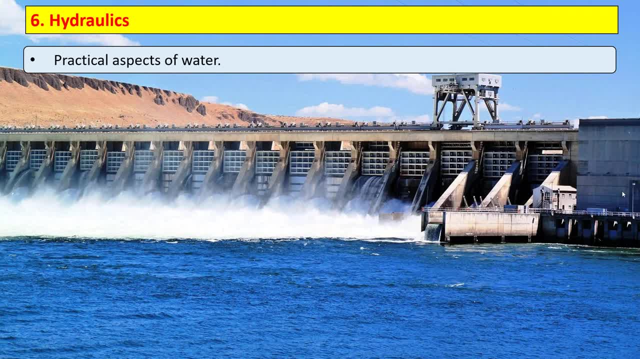 water. We can say it is a branch of science in which the study of fluids, liquids and gases at rest and in motion is done. Usually the liquid is water and the subject is titled hydraulics. When the water is at rest, the forces exerted by the water and immersed areas are found out. 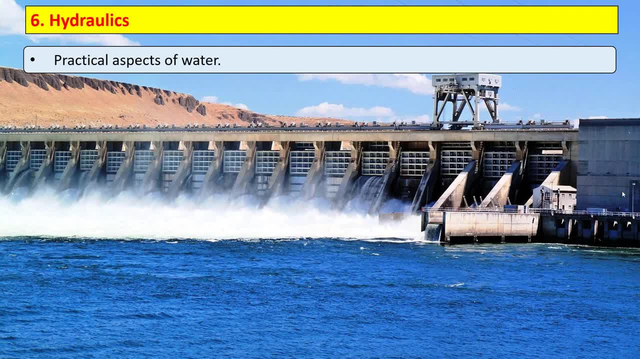 by the laws of mechanics. Thus, the knowledge of these forces is useful in the design of the gates used to control the flood water in case of dams, When water is drawn off from a reservoir and conveyed through a closed conduits or open channels. 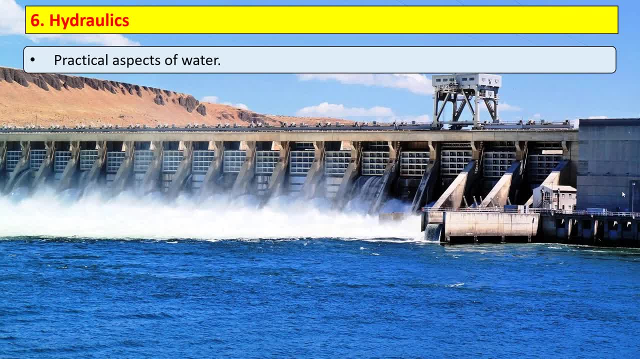 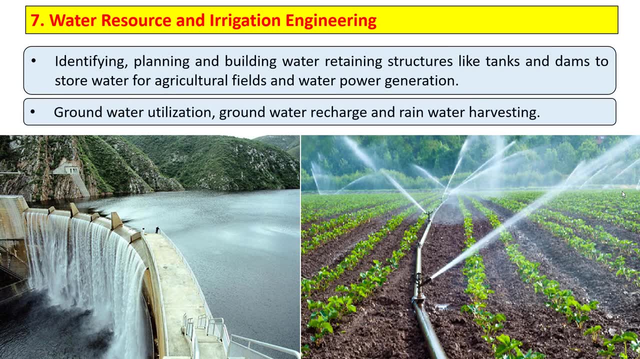 the knowledge of the behavior of the liquids in motion is also useful. Next, we have water resource and irrigation engineering. Mainly it deals with identifying, planning and building water retaining structures like tanks and dams to store water for agricultural fields and water power plants. Next, we have water resource and irrigation engineering. 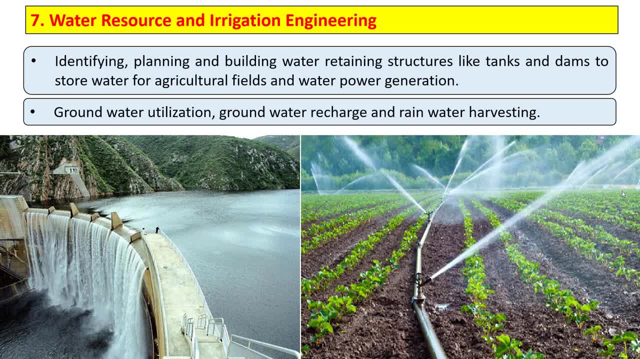 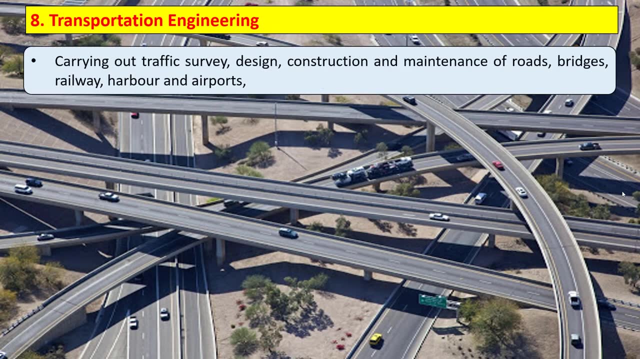 It is the main building of the flood water generation. Also, groundwater utilization, groundwater recharge and rainwater harvesting are the most important things in irrigation engineering. Next we have transportation engineering. It deals with carrying out tropic survey, design, construction and maintenance of roads, bridges, railway, harbor and airports. 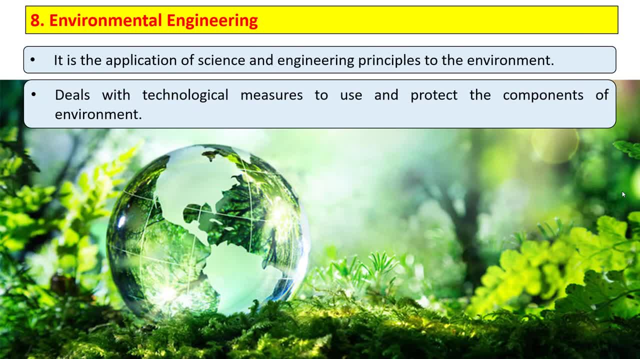 Next we have environmental engineering. It deals with the development of new solutions to flood water generation. Next we have environmental engineering. It deals with the development of new solutions to flood water generation. Next we have environmental engineering. It is the application of science and engineering principles to the 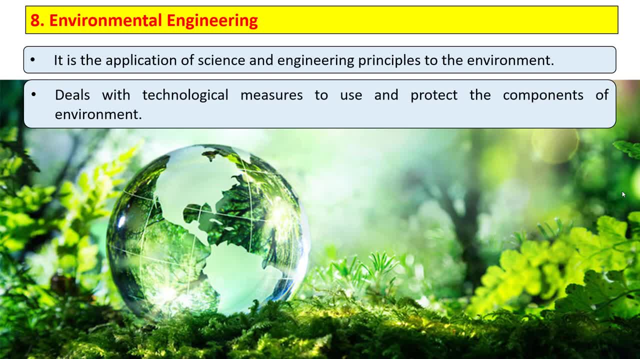 environment. It deals with technological measures to use and protect the components of environment. It is the important branch of civil engineering, which covers both water supply and sanitary engineering. The importance of clean environment was felt with the rapid growth in population and the growth in urbanization and industries. 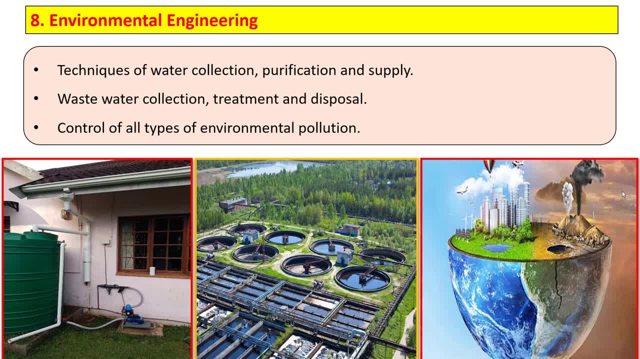 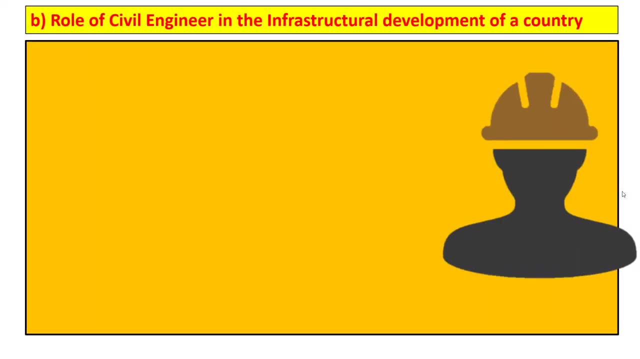 It is also environmental engineering. It also deals with the techniques of water collection, purification and supply, waste water collection, treatment and disposal, control of all types of environmental pollution. And the next concept, the second concept: what will be the role of the environmental engineering? It is the application of science and 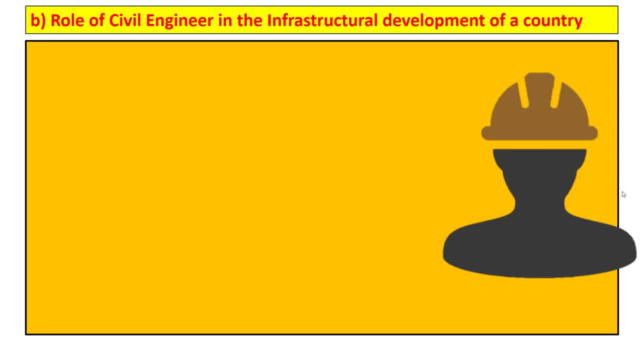 engineering principles to the environment. It deals with the role of civil engineer in the infrastructural development of a country, Like they are first of all. what do you mean by infrastructural facilities? The civil engineering constructions, electricity, telephone and internet facility, educational and healthcare facilities together we are going to call that. 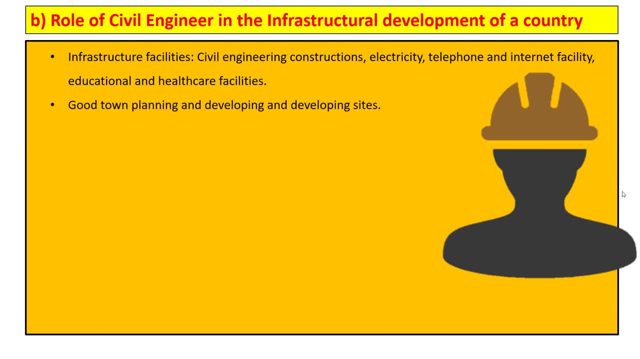 one as infrastructural facilities. What will be the role in that For a civil engineer? good town planning and developing and sites. then construct and maintain: road and railway network construction, development and maintenance of docks, harbors and airports to provide better irrigation facilities, the construction of dams and network of canals. 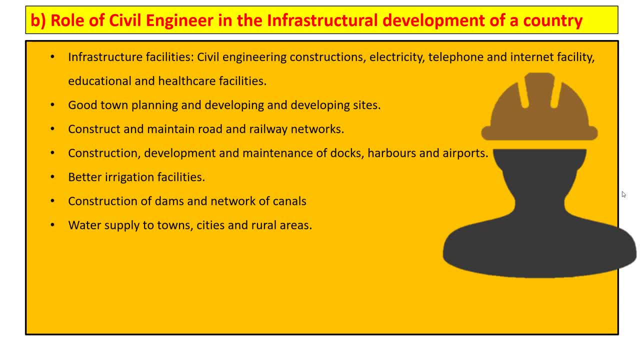 water supply to the environment and the construction of dams and network of canals, The design of good drainage and waste disposal system, solutions to environmental pollution and hazards. The most important thing is the careful planning and proper utilization of funds invested in infrastructural development to realize the maximum benefit. It will be the important part of the 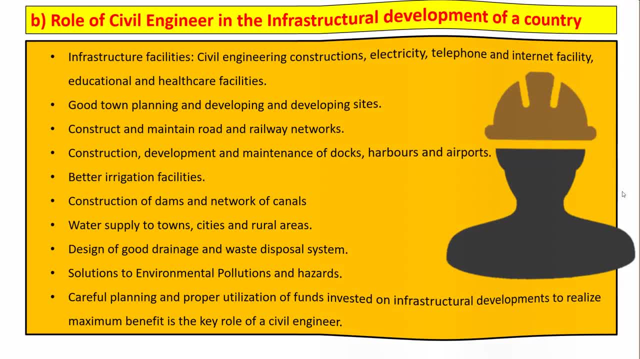 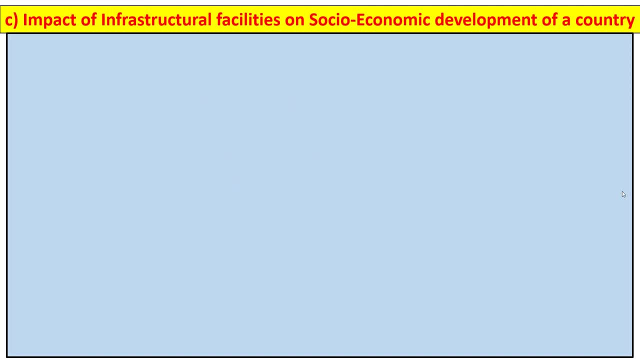 risk management and income management for a civil engineer. This is regarding infrastructure development And the last concept we have: what will be the impact of infrastructural facilities and social economic development of a country? It generates scope for lot of industries, the imports and exports. 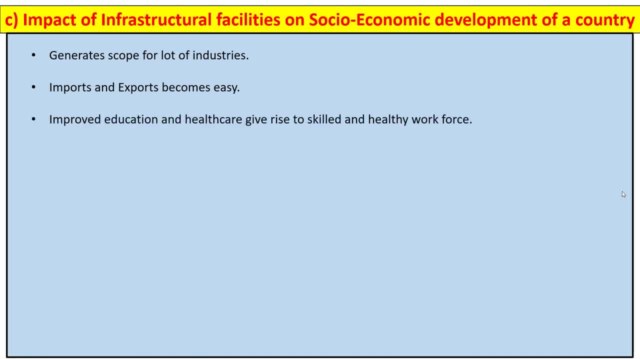 will become easy. Income and Exports will become easy. Income and Exports will become easy. Importance and export will become easy. Importance and export will become easy. Improved education and health care gives rise to skilled and healthy workforce, Increased in food production and protection from famine. like any disaster, 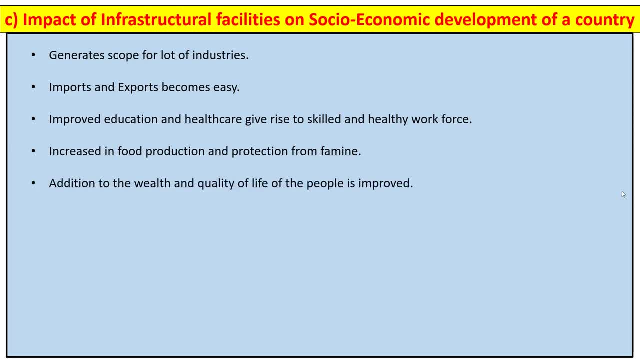 Addition to the wealth and quality of life of the people is improved. In case of the natural calamities, assistance can be extended easily and affected people are saved. The defense system can be improved and the peace will exist in the country by developing the infrastructural facilities.